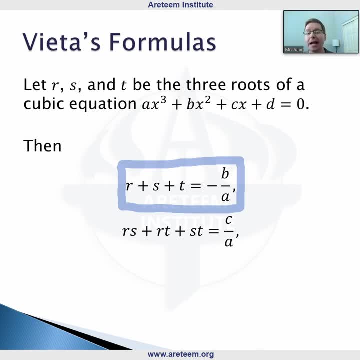 equation. When we had a quadratic there were two roots, so now our second term is two roots multiplied together all the possibilities. So R times S, R times T, S times T and those three values are added up and that's. 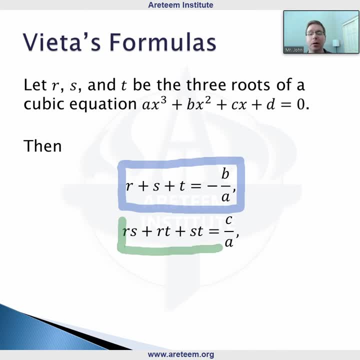 what gives us our C over A. So we have: the sum of the roots is negative, B over A. The sum of the product of two of the roots is C over A. Now what is our third term? Well, we have single roots, double sets of roots and then now all three of the roots. 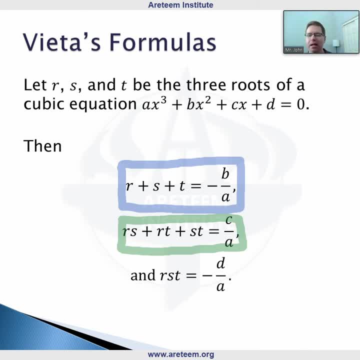 put together. So our third formula is: the product of the roots R, times S, times T is negative D over A. So this is kind of an extension of that quadratic. We'll see in future videos that this works for higher degree polynomials as well. but 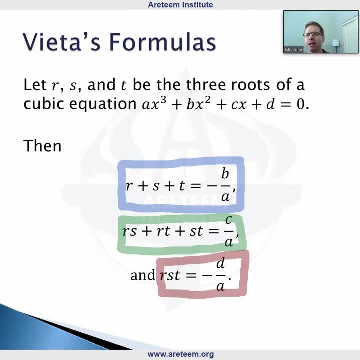 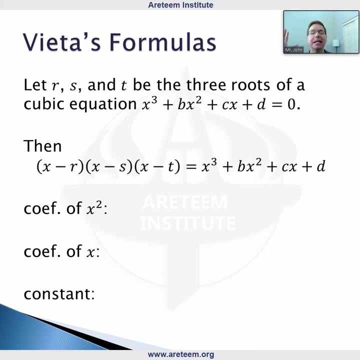 let's explore this cubic one and actually look at an alternative way of going through the proof of this. So looking at our setup here. So let's say we have our three roots. Notice, here I'm missing an A. You can, of course, just divide by A if you want to get rid of that. 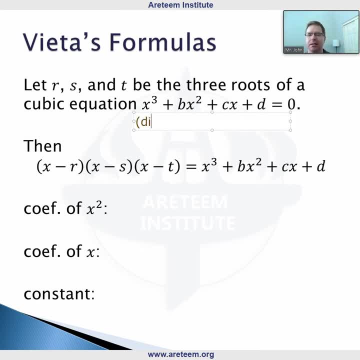 coefficient of the X cubed. So we can divide by A first, and then that gives us X cubed plus BX squared plus CX plus D. Doesn't change anything, it just allows us to kind of do a simplified proof of this here. now, if we're given the three roots that 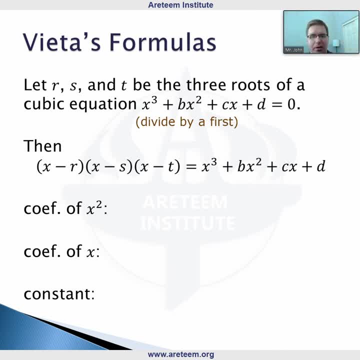 is a clue about how this would need to factor right. if R S and T are the roots of the equation, that means it's definitely going to need to factor with R S and T. this is the reason that we wanted to get rid of that a term, so we 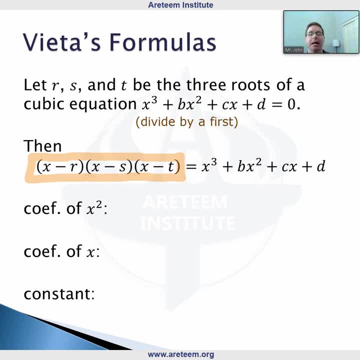 have just X minus R, X minus X, S minus X minus T. now this of course cannot actually change our equation, right? this has to still be equal to our cubic polynomial, X, cubed plus BX, squared plus CX plus B. right factoring it doesn't change anything. so if we start looking at this right, of course, multiplying this, 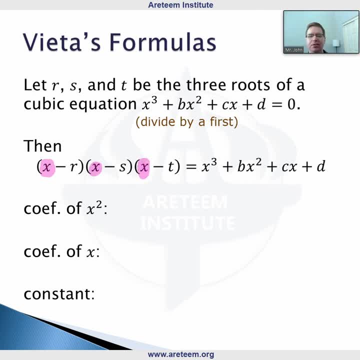 out: X times X, X times X x. that's going to give us our x cubed right. So that's how that first term will come up in that case. Well, what if we start looking at other terms from that? How can we get things like an? 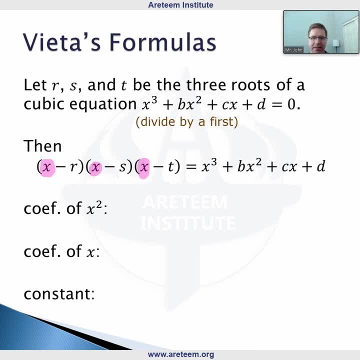 x squared. Well, if we have two x's and then minus t for the third term, right? So we have x times x times minus t, that's going to give us some expression with an x squared, right? So this is going to give us a minus t in that case, right? Well, what if we have the first and third x's and 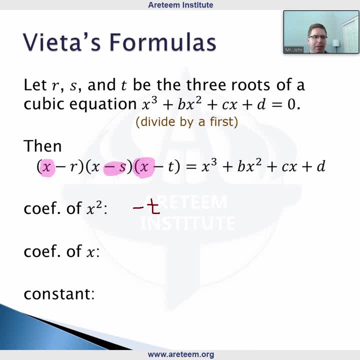 then we have a minus s for our middle term. Well, that's going to give us a minus s, of course, still x squared, right? So minus s, x squared. but if we're just looking at the coefficient, that is just going to be a minus s. Well, we also have then a minus r here as well. So minus r. 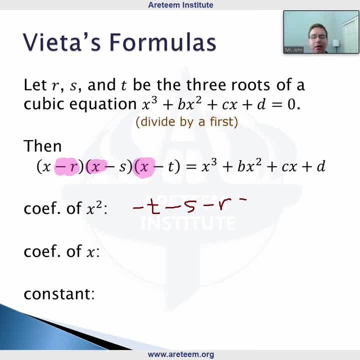 and this is our coefficient of x squared. So this is supposed to be b right Now? notice this is almost exactly our expression. We're supposed to have negative b over a right. A is one in this case. So if we make all of these things positive, 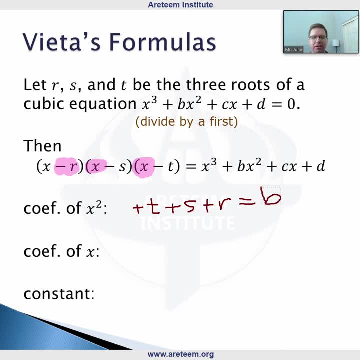 right. So we're supposed to have negative b over a right. So if we make all of these things positive right, So if we make all of these things positive right, So if we make all of these things right, plus r, plus s, plus t, this is going to be giving us a negative b in that case. So 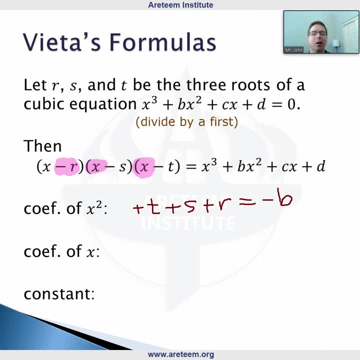 right, negative. b over a, basically, is the sum of the roots there, And this is the game we can play for all of the terms, right, We can do some of these a little bit quicker in this case. Well, what if we just want a linear x, right? Well, we could have negative, r, negative. 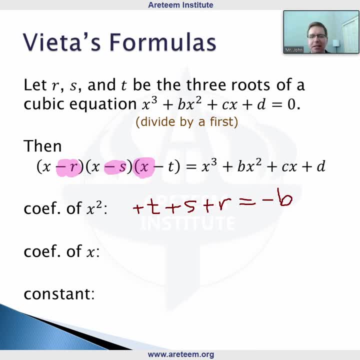 s times x. So that gives us a positive r s. in that case, right, Then right, what if this middle term is the x? right? So then we have negative r, negative t times x, So that is plus r times t. And finally, right, we look at negative s and the first term is our power of x. 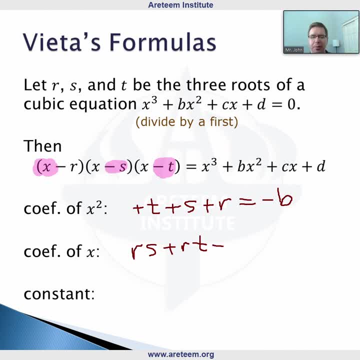 x times negative, s times negative. t is plus st. No negatives to worry about here. This is supposed to be our c value. Our linear term has a coefficient of c, So we have c over a because we divided by that a first. Now, when a is: 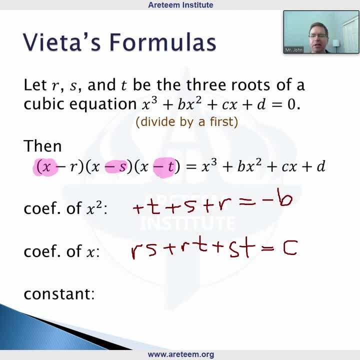 one, it is just c. Very similarly here, what is our constant term? The only way to get the constant is negative r, negative s, negative t. So we have negative r s, t is equal to d, And then, moving that negative over, we of course just: 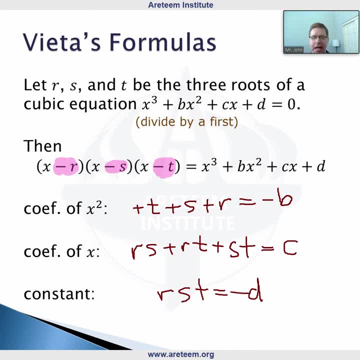 have our r? s? t is negative d, as we needed in that case. right, So that gives us our value that we want there. Some of the roots is negative b or negative b over a, If you have the a. 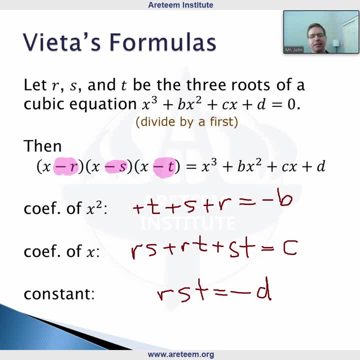 the sum of the product of two of the roots together is c or c over a, And then the product of r, s and t, all three of the roots put together- is negative d or negative d over a in the general case, And that idea of the proof can be extended further as 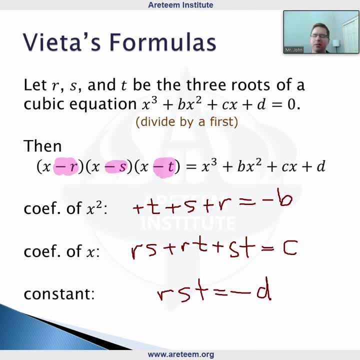 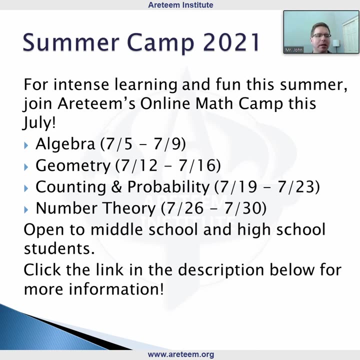 well to higher powers and higher degrees of polynomials, which we'll explore in a later video. In this video I want to make a special announcement. So this Vieta's theorem formula here is a great formula that you will see in a lot.